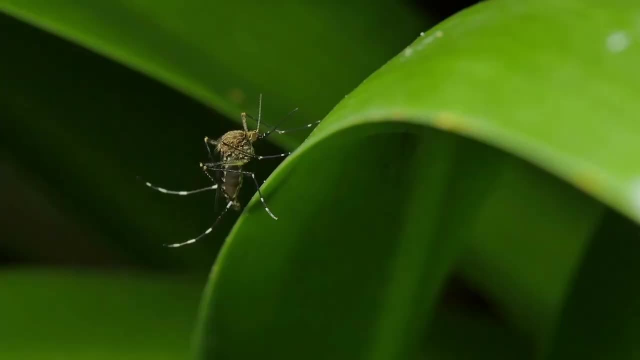 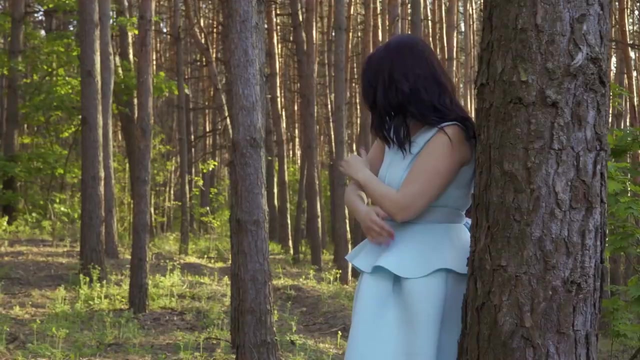 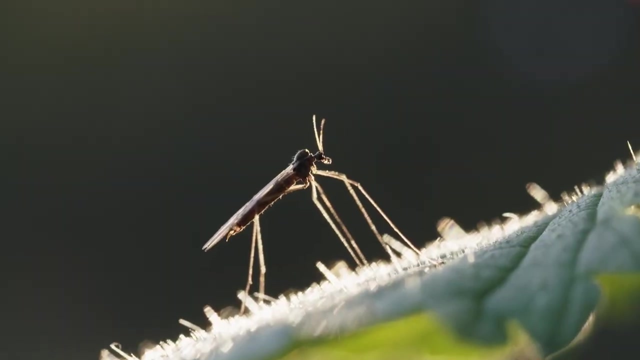 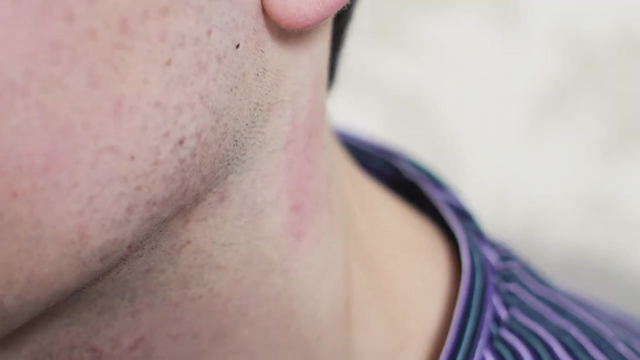 But there is one type of insect I am not a fan of – mosquitoes or, as Australians like to call them, mozzies. Their bite can ruin your picnic and their annoying buzz can keep you up at night. Most importantly, some mozzies can spread diseases like malaria and dengue fever. 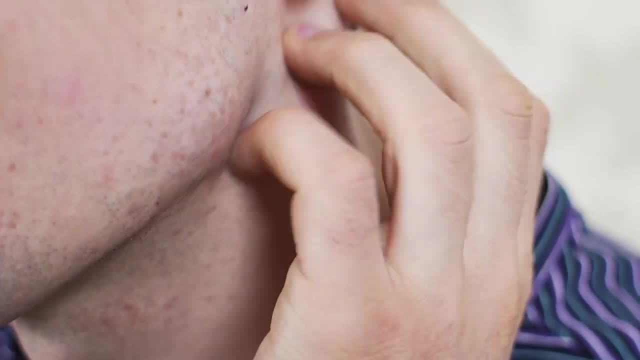 To help prevent the spread of the disease. you can use a mosquito repellent To prevent the spread of the disease. you can use a mosquito repellent To prevent the spread of these diseases and control mosquito populations. it's important to learn about their lifecycle. 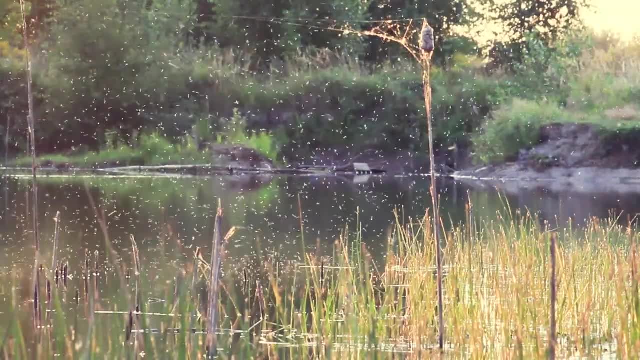 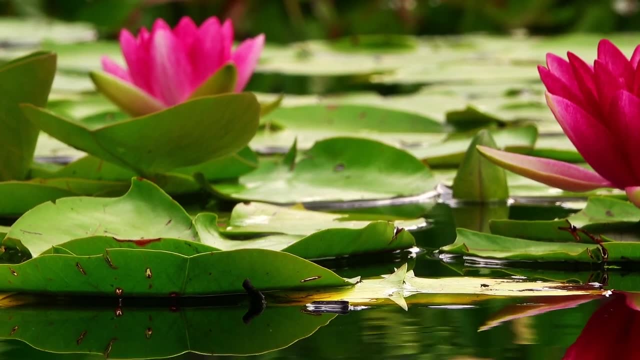 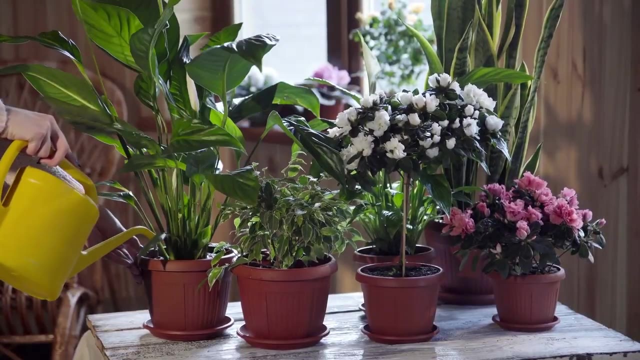 So let's take a look. In order to reproduce, mosquitoes need fresh water that is stagnant. Stagnant means the water is not flowing like the water in ponds, puddles and around the base of plant pots. After mating, a female mosquito lays eggs in water. 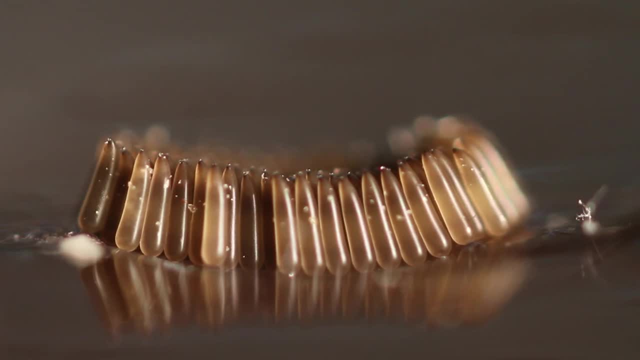 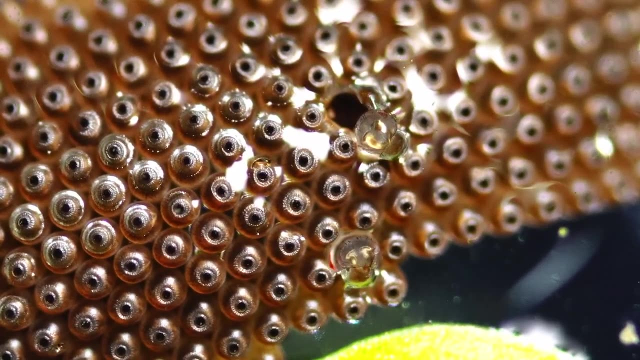 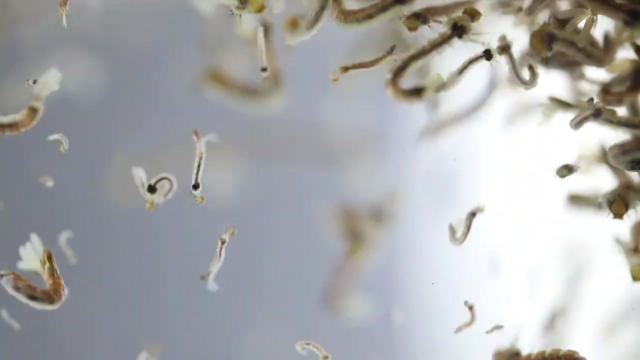 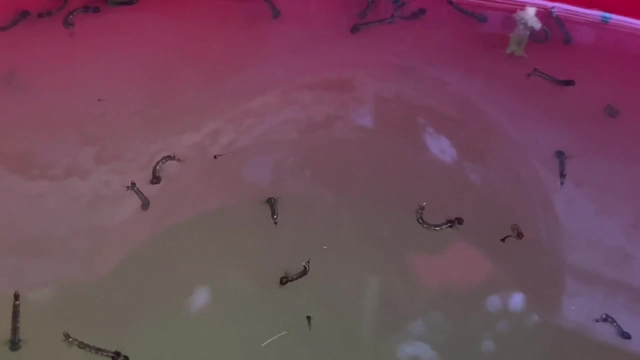 The eggs are grouped together, forming an egg raft. A mosquito larva hatches from each egg. The larvae do not look like adult mosquitoes at all. They have elongated bodies that hang at the surface of the water. They get the oxygen they need by taking in air through a snorkel-like tube called a siphon. They get the food they need by filter-feeding on microorganisms around them. To escape danger, larvae will often dive below the surface in an S-like motion, which is why they often get called wrigglers. The larvae molt and grow rapidly, with the whole larval stage lasting around 10 days. 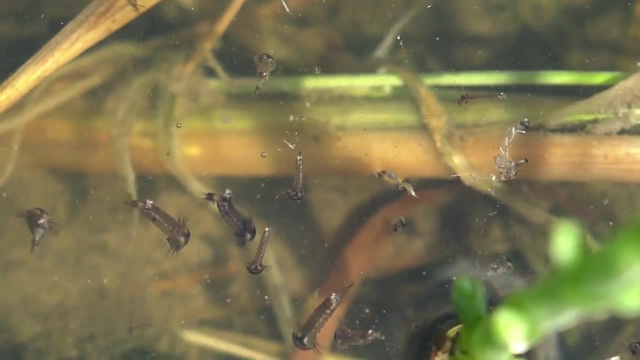 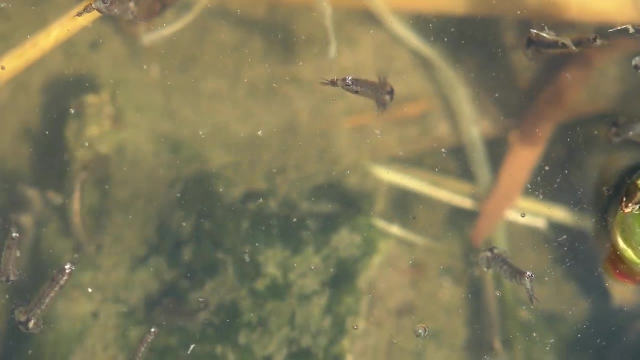 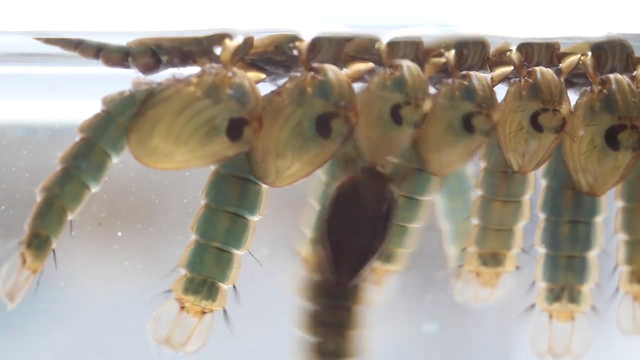 Next up, the mosquito enters the non-feeding pupils. The pupae still require oxygen and take in air at the surface of the water. Pupae are sensitive to changes in their environment and respond by rolling below the surface, giving them the nickname tumblers. 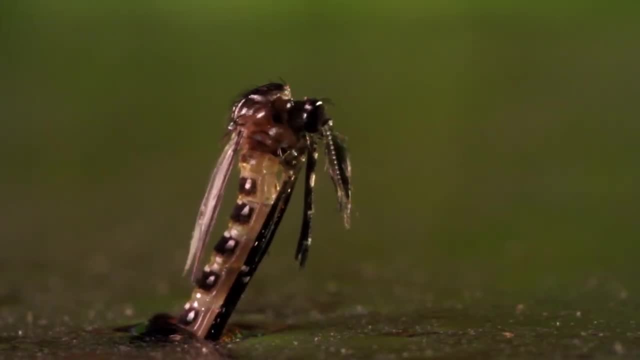 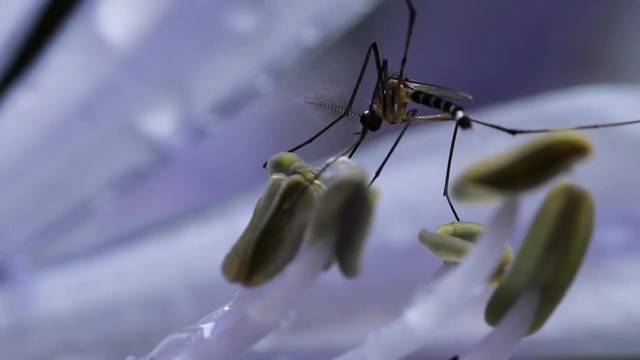 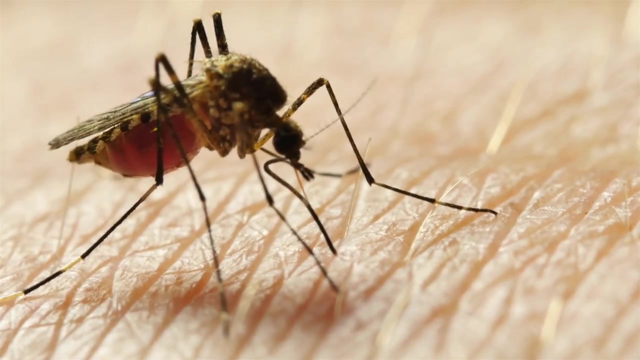 The pupal stage lasts for just a few days, after which an adult mosquito emerges. The pupal stage lasts for just a few days after which an adult mosquito emerges. Male adult mosquitoes usually feed on nectar from flowers. Female adult mosquitoes feed on the blood of humans and other animals.